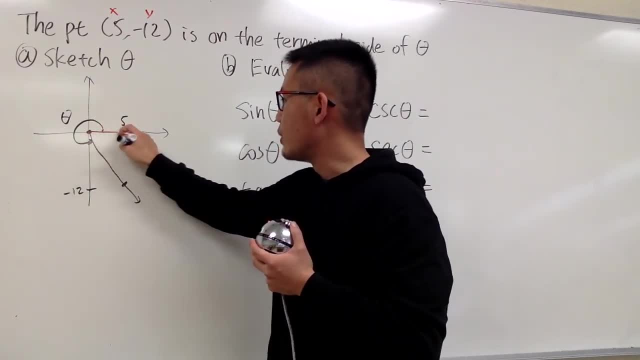 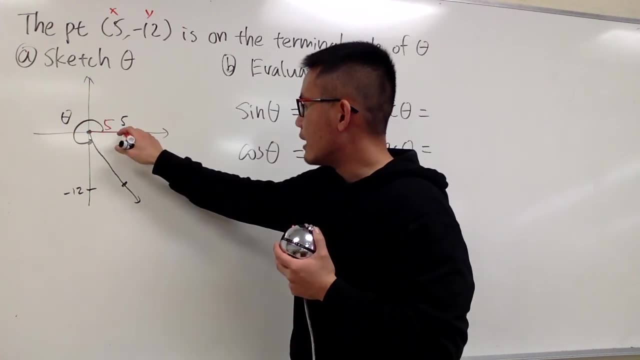 You see that from the origin to 5, the horizontal distance is just the x value, it's just the 5, right? So let me put this down as 5.. And we also know that, if you just go down right here, that's the y value. 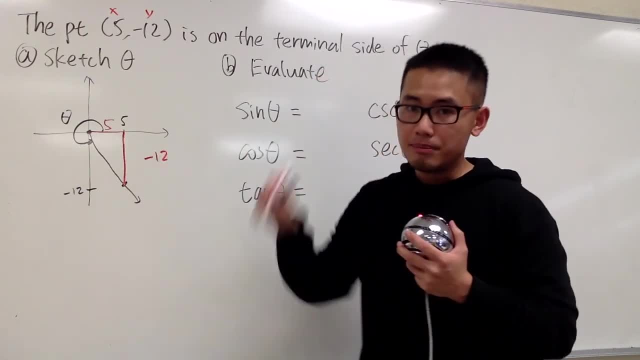 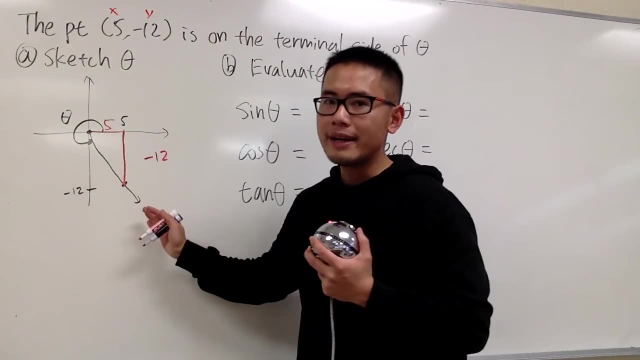 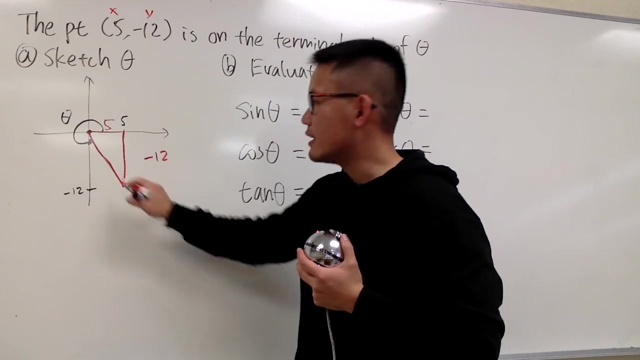 and we know that's technically negative 12, because that's down below right. So you label this side as negative 12. And we pretty much have a right triangle already. But one more thing that we need: We also need to know the hypotenuse from here to here of this right triangle, isn't it? 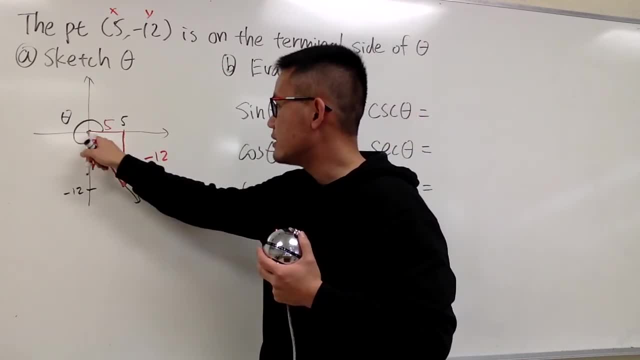 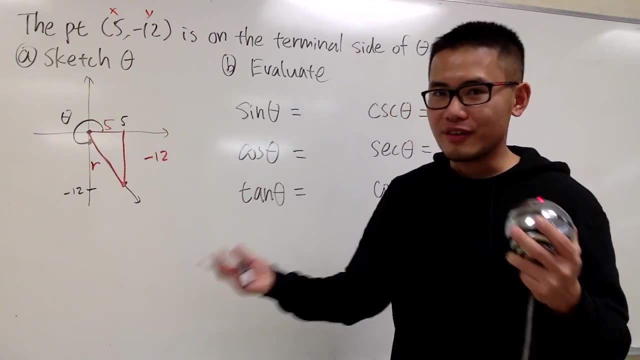 And in this situation we'll label this as r, the distance from the origin to this point. And we have a formula for that. It's pretty much just the parsecron theorem. but we have the formula. It's just the. r equals to square root of x squared plus y squared. 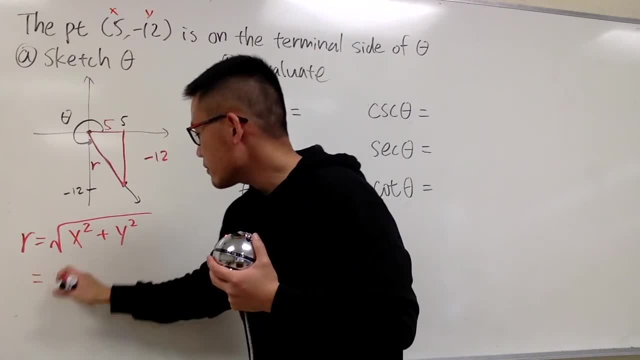 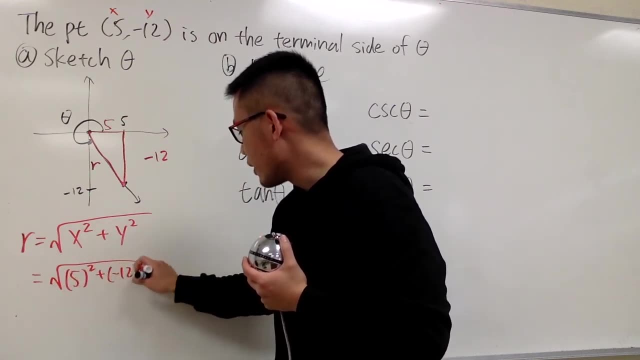 And let's just go ahead, put everything in and work this out. This is going to be: x is 5, so we have 5 squared plus the y value is negative 12 squared, And we have 5 squared is 25.. 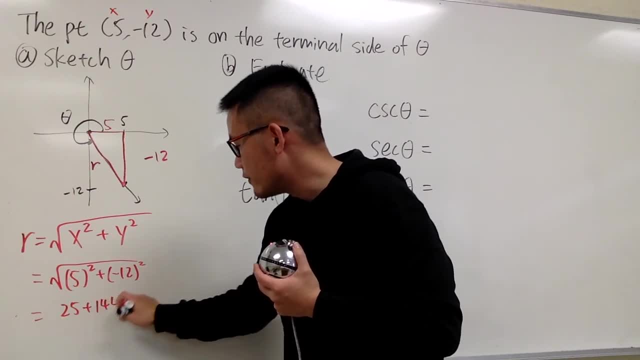 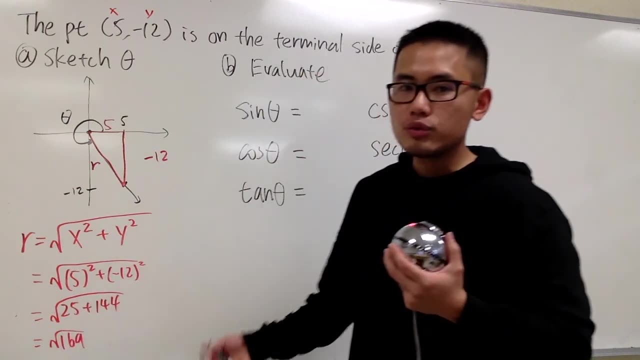 And then we add it Negative 12, and then squared is positive 144.. We take the square root for that. After that, this is square root of this, and that together is 169.. And square root of 169, we know this is going to be 13,. right? 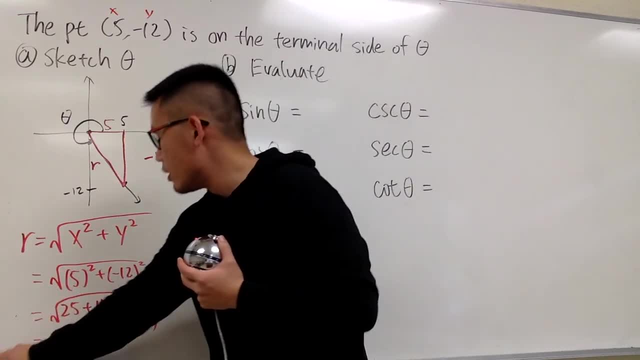 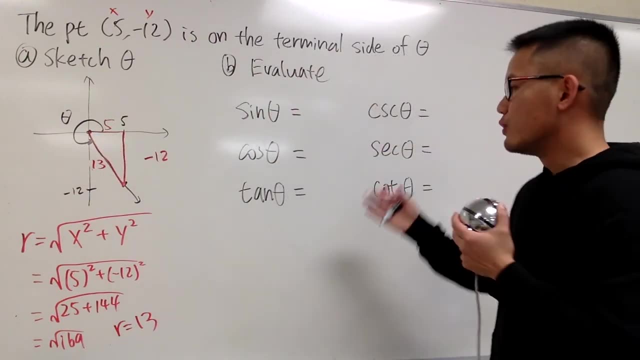 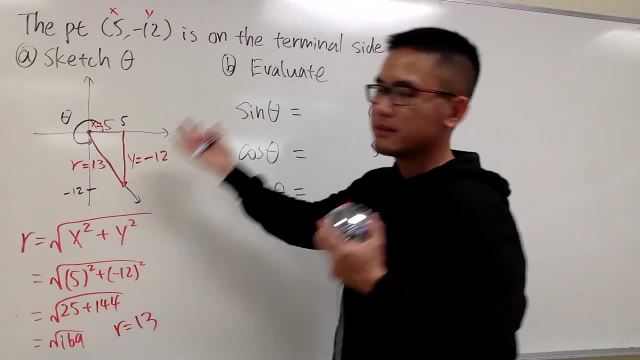 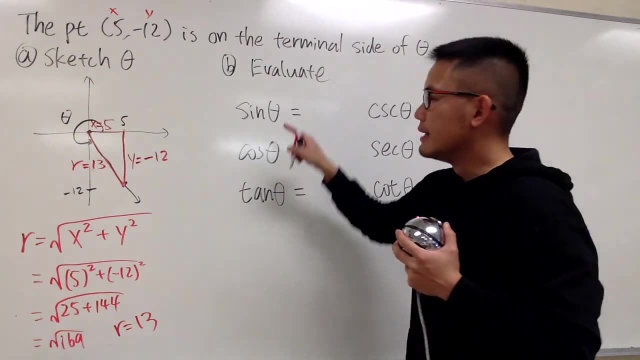 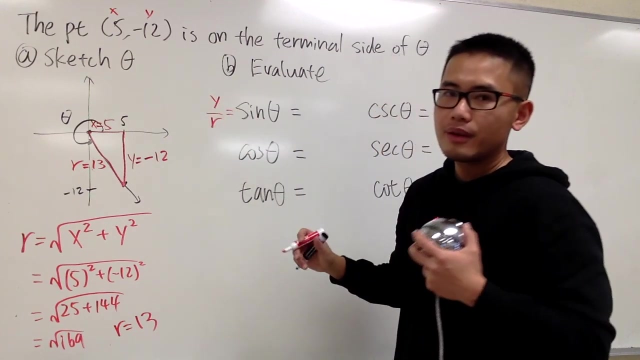 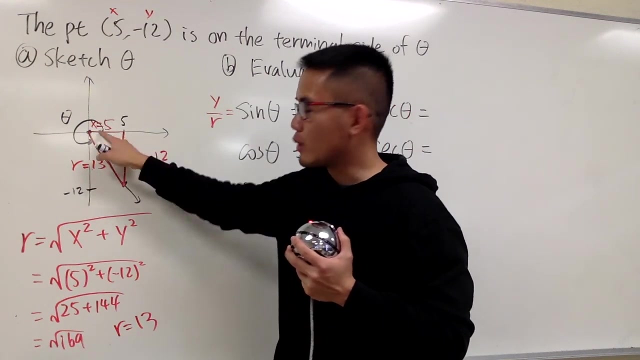 is negative 12 and the R is 13, just to make this super clear anyways. so these are the things for to remember in this situation. sine theta is defined as Y over R. okay, why is this technically, if you look at this as your reference angle? okay, this part right here, because we are talking about right triangle. sine it's. 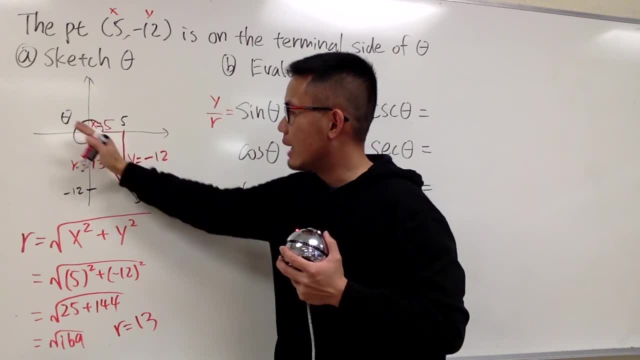 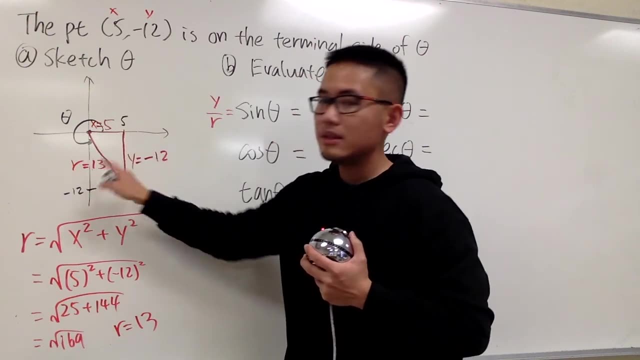 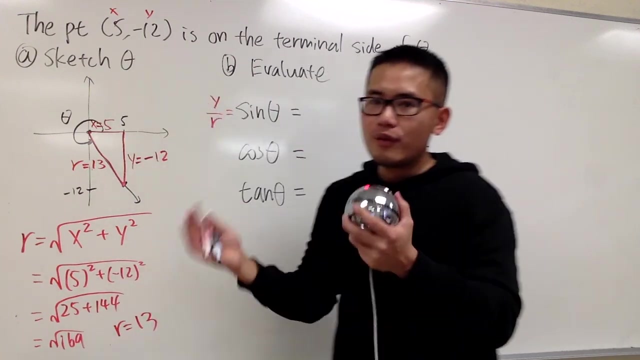 the opposite. right, it's the opposite over the hypotenuse. that's exactly why is Y over R? so here is the opposite, and the hypotenuse is 13 and, by the way, R is always positive. keep that in mind, X and Y. of course, it can be negative, or 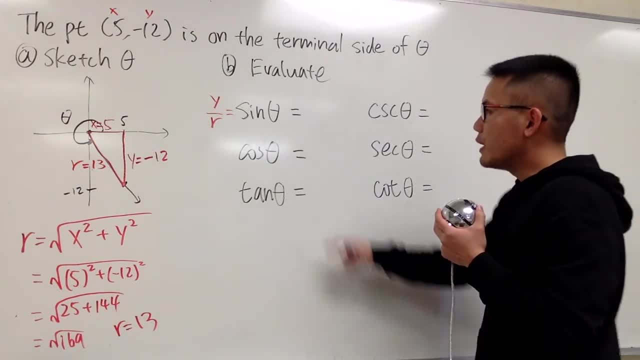 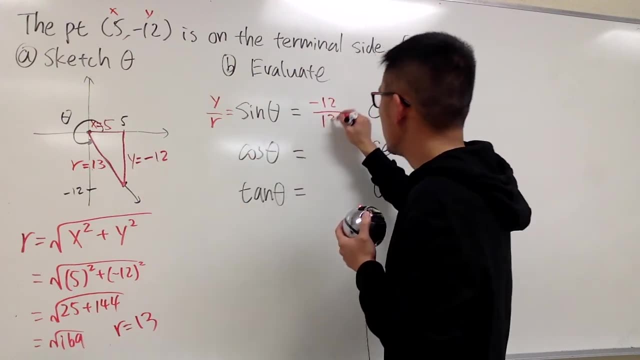 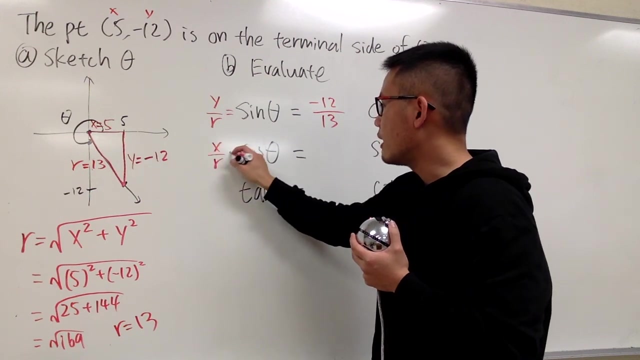 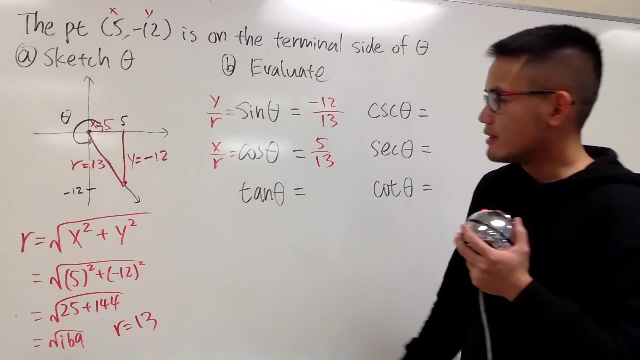 positive, but R is always positive. okay, anyways, sine theta is Y over R, which will have negative. 12 over R is 13, and that's it. and then cosine theta will find this kind of definition: it will be X over R and the X is 5, R is 13. so the answer to this is just 5 over 13 and for tangent, 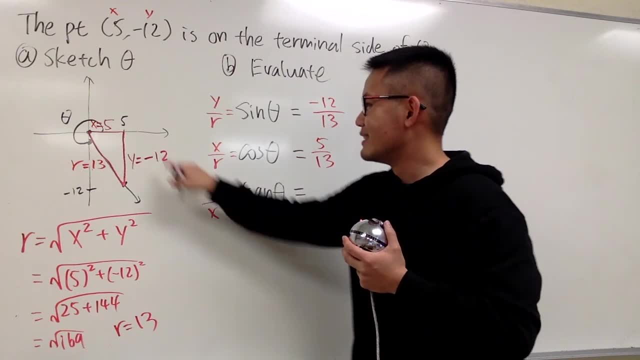 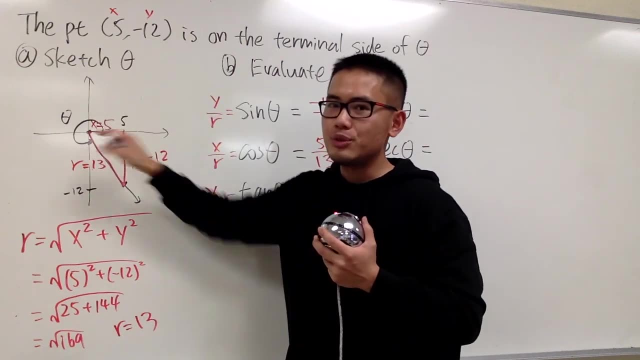 is what? Y over X, Y over X, it's just the same as opposite over adjacent. all right, if you look at this as your reference angle. anyways, Y is negative 12 over negative 12 over R is negative 12 over R is negative 12 over R is negative 12 over. 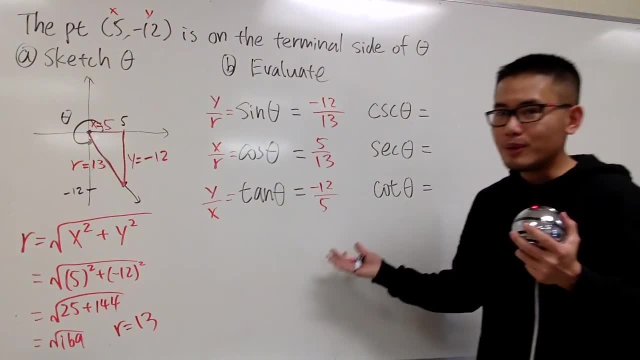 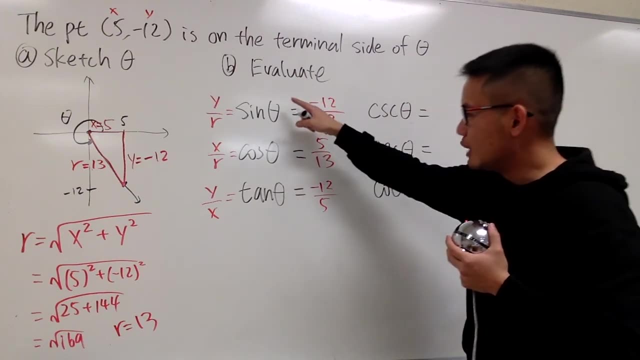 negative. 12 over R is negative, 12 over R is negative, 12 over R is negative, 12 over X, which is 5. and this is pretty much it for the three famous one sine cosine tangent of the angle theta, because once you have this three done this right here, 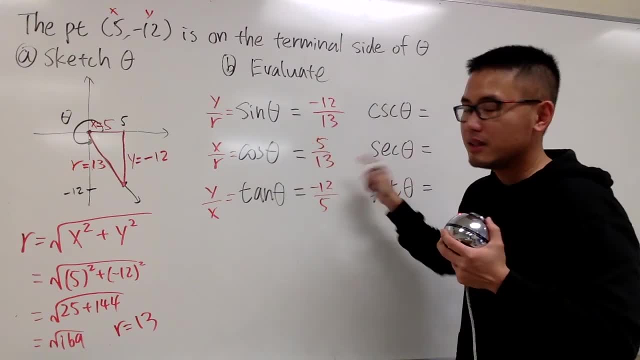 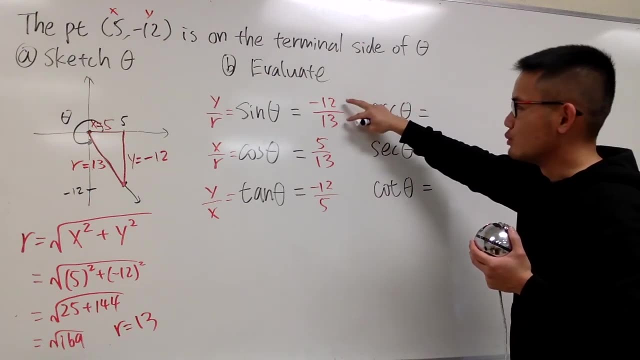 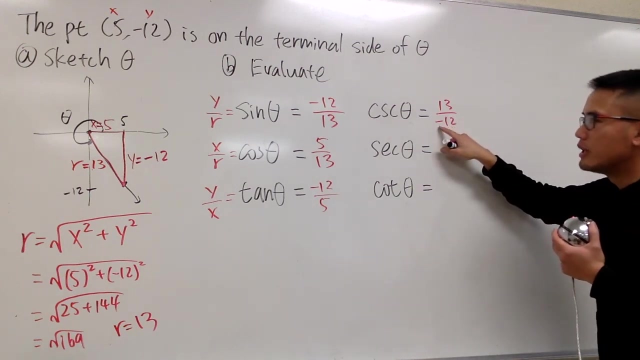 are pretty much for free, because if you set this up correspondingly, sine theta, cosecant theta- you know the relationship of this and that is: you just flip this right, you do. the reciprocal cosecant theta is just you flip that which is 13 over negative 12. of course, you can put it on the other side of the equation and 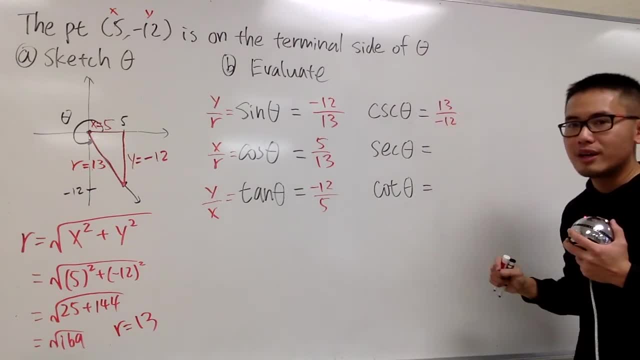 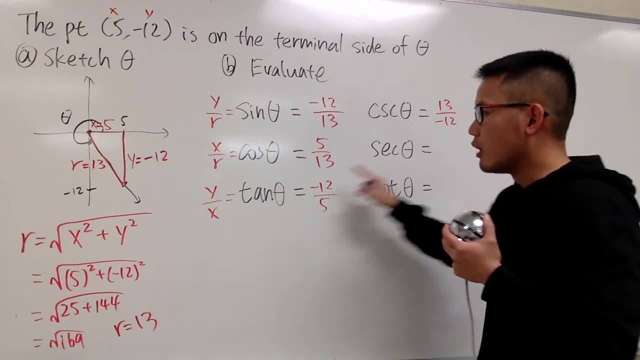 put the negative in the front. well, on the top doesn't matter, but let me write it down this way. next we have secant theta, which is just a flip of that. secant theta is just a reciprocal of cosine theta. okay, so we'll just turn this into 13 over 5.